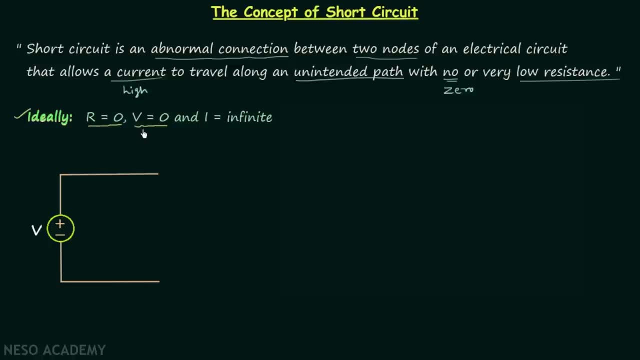 zero ohms and the voltage or the potential difference across the unintended path is equal to zero volts, but the current is equal to infinite. it is infinite because resistance is equal to zero. let's understand this by the help of one example. in this example, I have taken one voltage source. we are 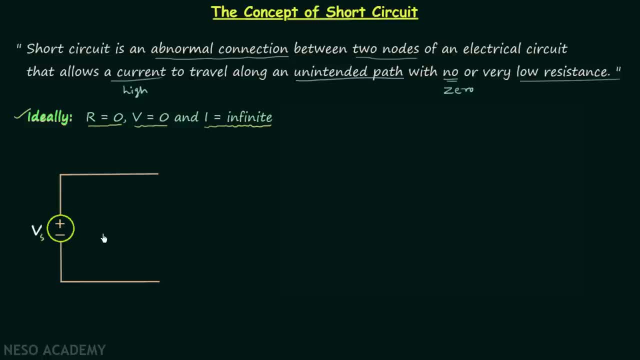 having one voltage source vs. and the voltage source is having the positive terminal here and the negative terminal here, and let's say, by any means, there is an abnormal connection between the positive terminal and the negative terminal. and due to this abnormal connection between these two nodes, which 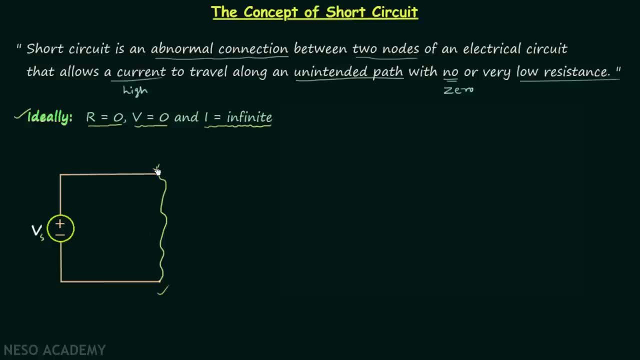 are at the different potentials. there exists an unintended path and this unintended path will have the resistance equal to zero ohms. and from Ohm's law we know the current I is equal to voltage, which is Vs in our case, divided by the resistance, which is equal to zero. so from here we are getting. 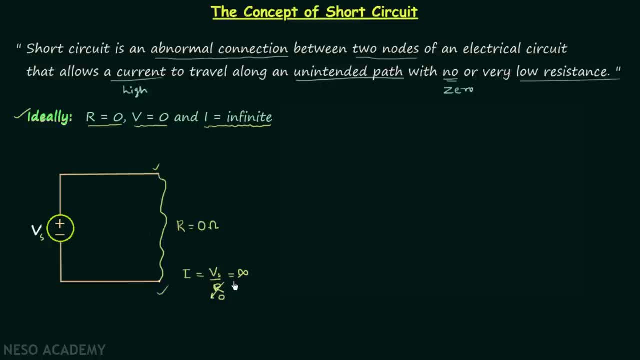 current I is equal to infinity, so a very high current will flow through the unintended path, or you can say in this circuit, and due to this very high short circuit current, a very large heat is produced in the circuit and, practically speaking, this circuit is not possible. this is not possible because this 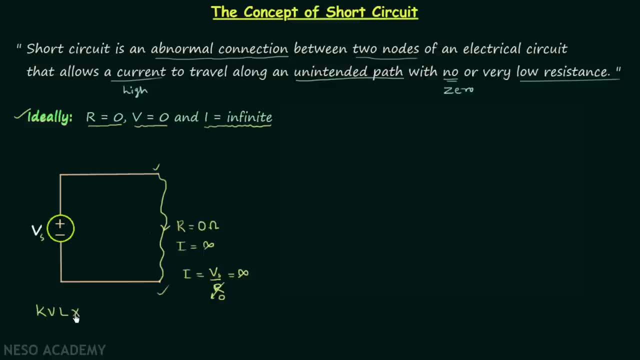 clearly violates KVL and KVL is based on law of conservation of energy and as KVL is violated, law of conservation of energy is also violated. so ideal case of short circuit is not possible and current will not be infinite. now we will move on to the 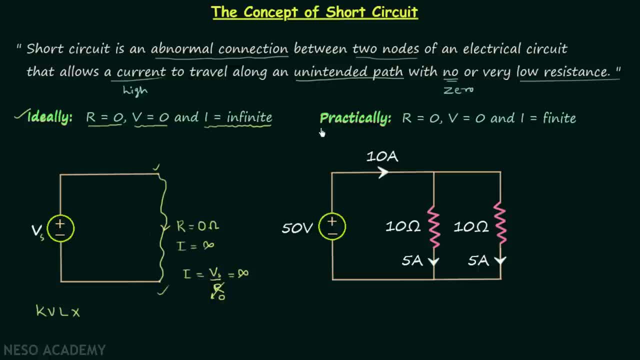 practical case of short circuit. and in practical case the resistance of the unintended path is equal to zero ohms, same as the ideal case, and the potential difference or the voltage across the unintended path is zero, same as the ideal case. but the current is not infinite, it is finite. 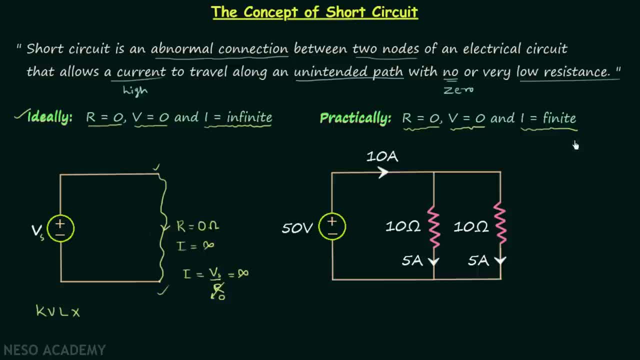 now we will take one example to understand this in a much better way. in this example, we are having a voltage source equal to 50 volts and two resistances are connected in parallel, and both the resistances are same. 10 ohms are the values of the long circuit and the resistance is equal to 0.5 ohms. 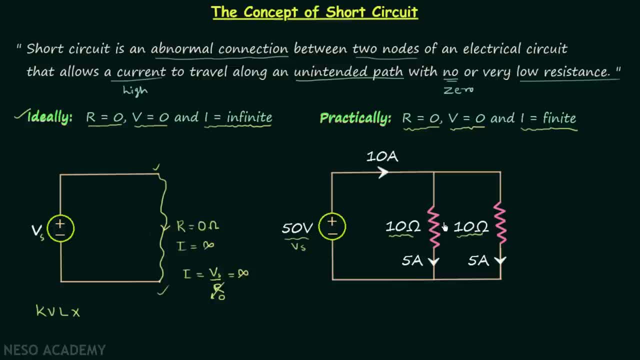 and the current is not finite. it is finite. now we will take one example to understand values of the resistors we are using in parallel and they will draw current equal to 10 amperes and the current will divide equally and therefore 5 ampere current will flow through this resistor. 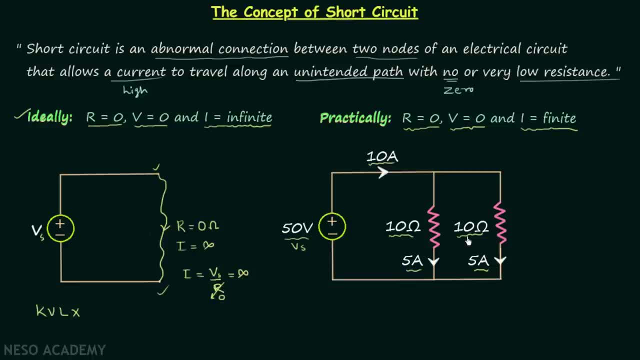 and 5 ampere current will flow through this resistor as well. Now, let's say, due to some reason, these two nodes are connected abnormally and therefore there is an unintended path between the two nodes which are at the different potentials, and the resistance of the unintended path is equal. 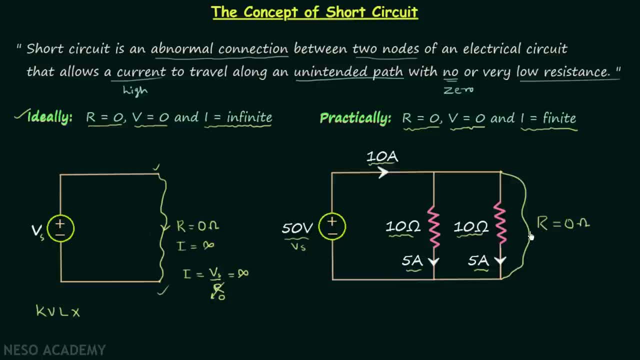 to 0 ohms and in both the cases voltage across the unintended path is equal to 0 volts, because these two Nodes are connected directly and therefore there will not exist any potential difference. The potential at this point will become same as the potential at this point because there is a path having the zero resistance. 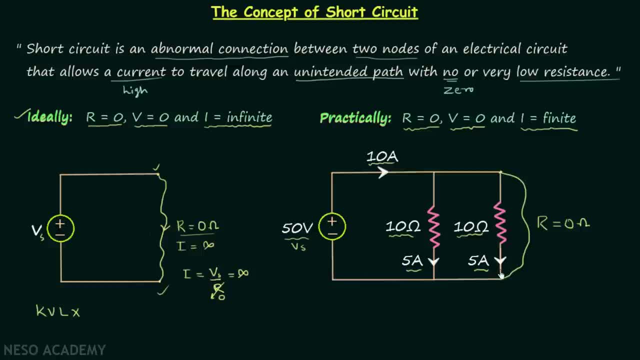 Similarly, in this case, this node and this node will have the same potential after development of the unintended path. Now we will focus on the current. Initially, the current was equal to 10A and as soon as the unintended path is developed, this 10A current will not divide it in these two paths, but it will directly flow through the unintended path.